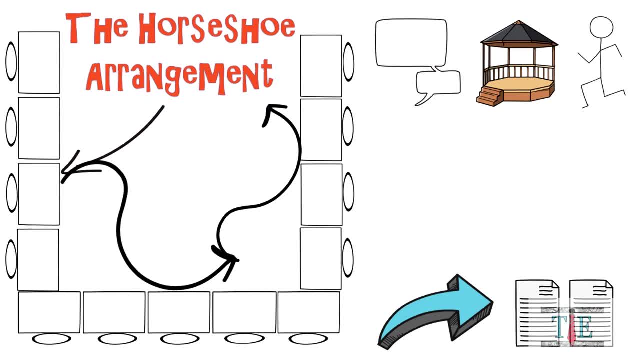 other out. On the other hand, this often leads to students copying one another's work. The Horseshoe Arrangement is good for discussion forums. Students can take center stage, Teachers can easily get to the students. The space can be used for kinesthetic activities, but students often copy each other's. 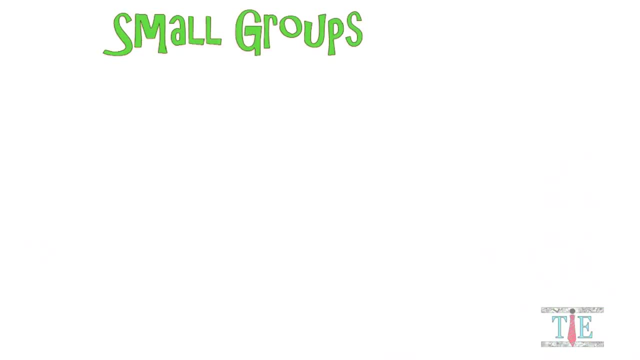 work. Now let's move on to the third seating arrangement, which is small grouping. This is sometime called group pods. Here the teacher's desk is usually located in front of the room. The student desks are situated in groups of four, although other variations are possible. The teacher can move. 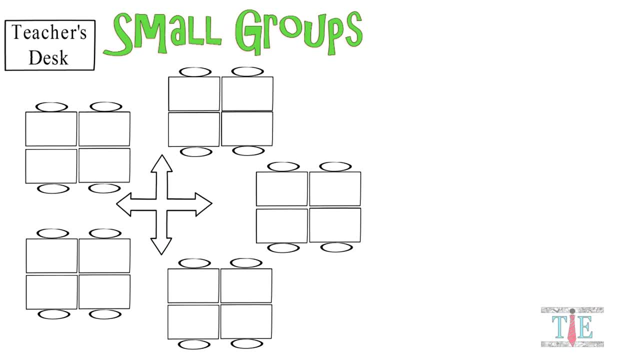 about freely and facilitate group learning. that's usually taking place. Small groups allow for cooperative learning and students can discuss project plans And they can work together as a functioning unit to develop teamwork skills. As the students are working on their projects, the teacher can walk around the room and facilitate learning. Some downsides include the room getting 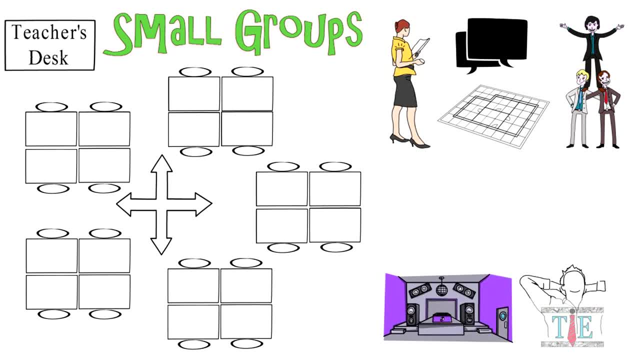 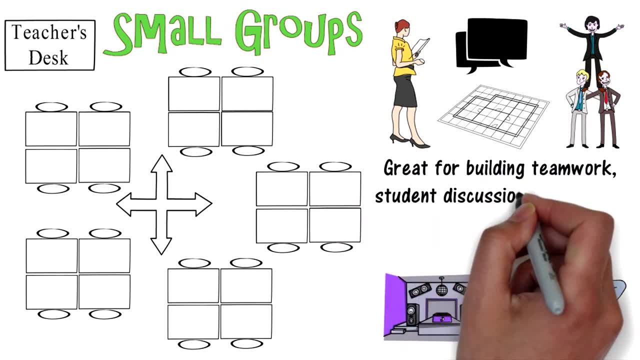 a little too noisy And with group work there's usually one person in the group that doesn't put their share of effort. So, to summarize, the small group arrangement is great to build teamwork, student discussions and doing projects, but it can get loud and not all students. 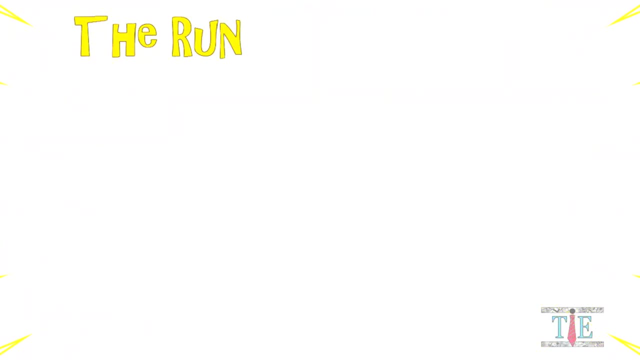 will contribute equally. The next classroom arrangement style is the runway. The teacher's desk is usually in the corner, students facing one another. This creates a large space in the middle of the room. Teachers will stand in the middle and bounce back into the calendar space. 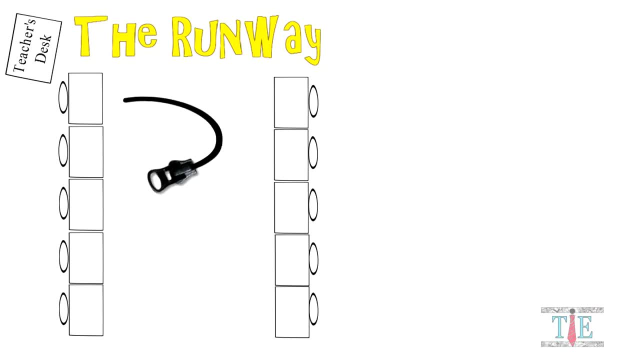 This creates a large space in the middle of the room. Teachers will stand in the middle and bounce back into the jibbyeway and forth from student to student. The runway is most often used when teachers are setting up a classroom debate. Each side of the runway will have their own. 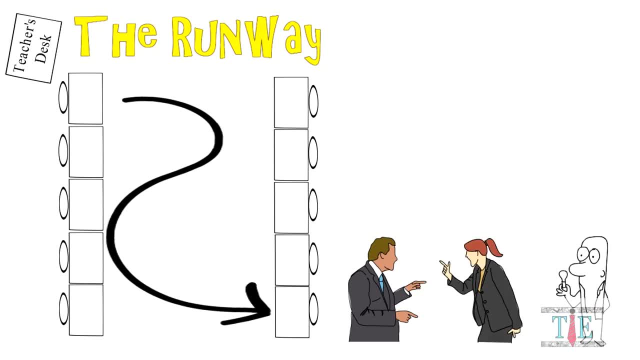 argument. Other times, teachers can use the open space to perform demonstrations for students. This arrangement does lead to students shouting across the room. So to summarize here, the runway is great for political debates. Students can bounce ideas off one another. However, it does get loud and students on the ends. 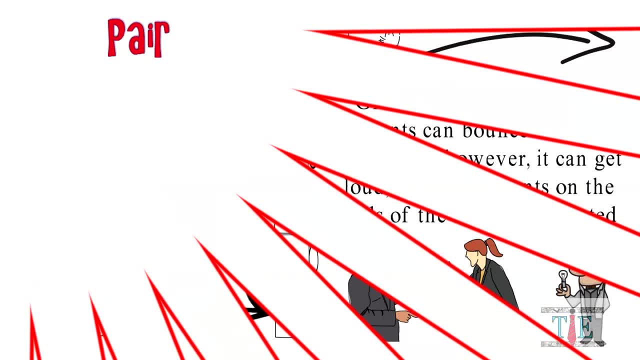 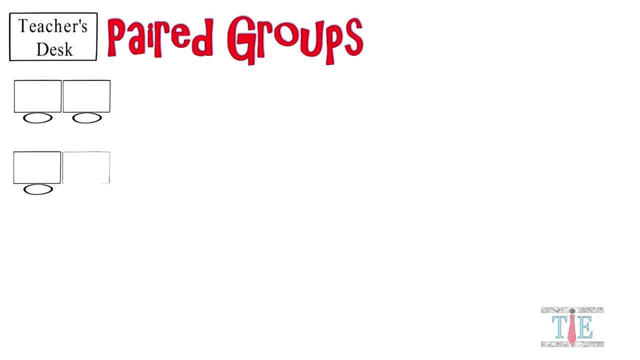 of the rows often feel isolated. The next arrangement style is called paired groupings, Although many other names exist, such as paired pods. the teacher's desk is located in the corner or front of the room. The desks are arranged in groups of two and they're facing the front of the classroom. Now, when it comes.